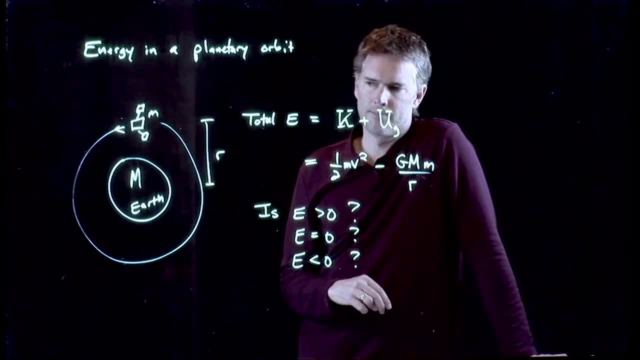 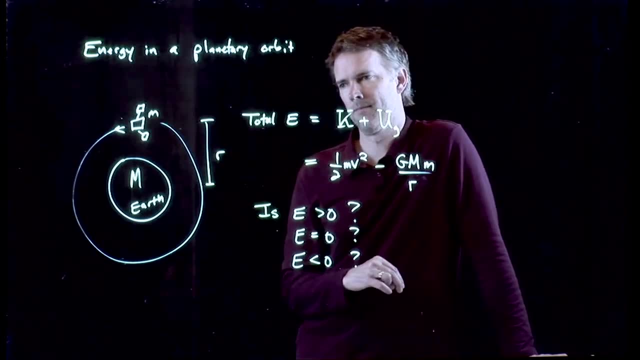 So let me ask you guys: What do you think, Jackie? what do you think? Is the energy going to be positive, zero or negative? Okay, excellent, That's why we're here. That's why we're here, right. 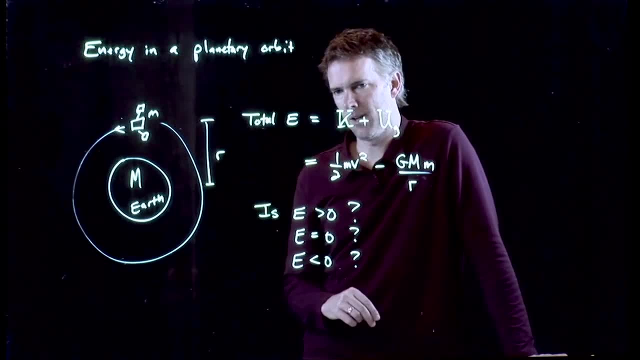 Yeah, If we knew all the answers, why would we be here? Okay, What do you think? Do we like the idea that things have positive energy, Or are we okay with the fact that they maybe have negative energy? You like positive? 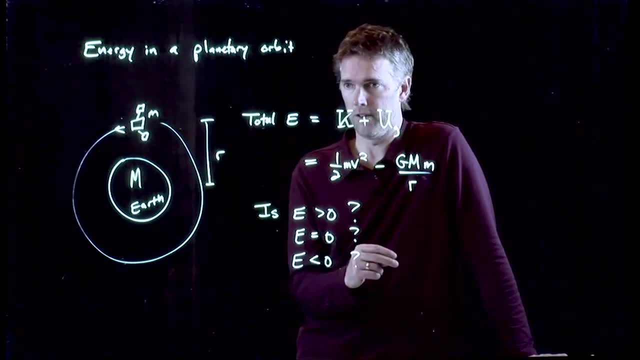 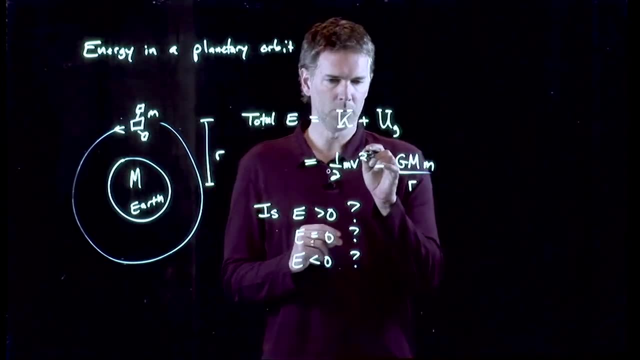 Not necessarily All right. So we don't know the answer to this right. Let's see if we can figure out. the answer to What we can do is we can relate this v to some of this stuff over here. Okay, how do we do that? 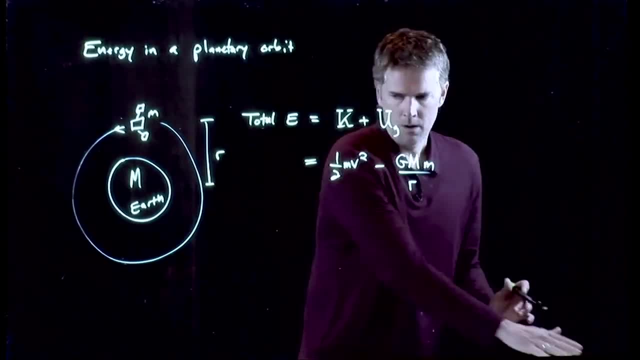 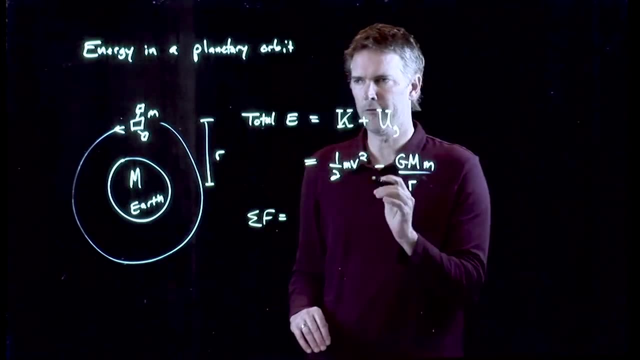 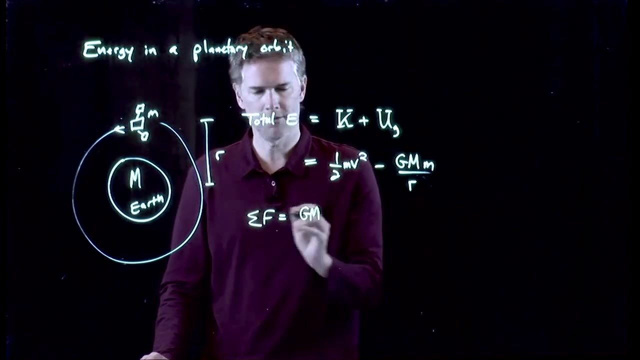 Well, what we remember is that if it's moving in a circle, the sum of the forces have to add up to mv squared over r, And there's only one force here, It's g: mass of the earth, mass of the satellite. 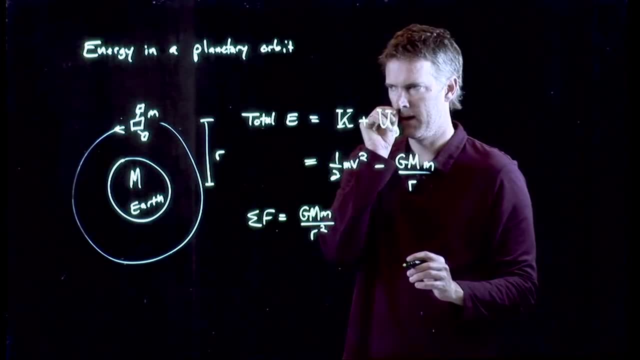 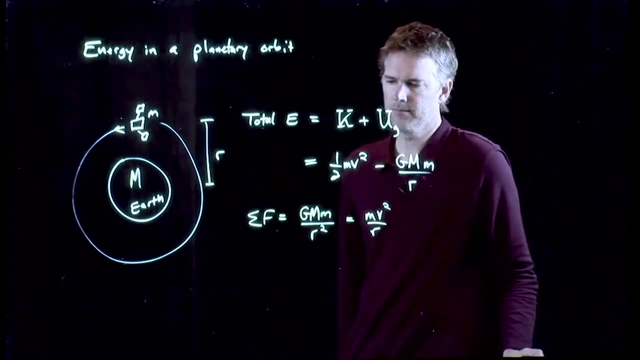 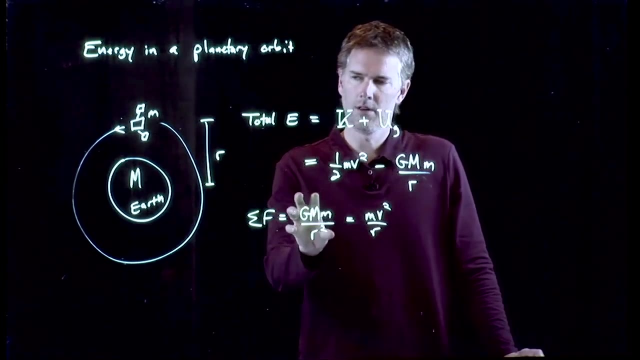 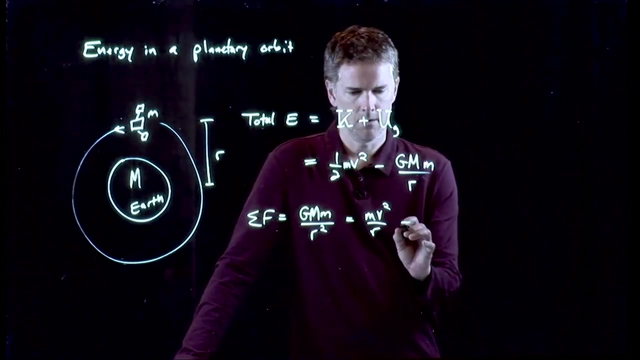 divided by r squared, That equals mv squared over r, And so it looks like I can relate this mv squared stuff to these other parameters, Which maybe we can solve this and plug it back into there. All right, What do we do? Well, let's multiply both sides by an r. 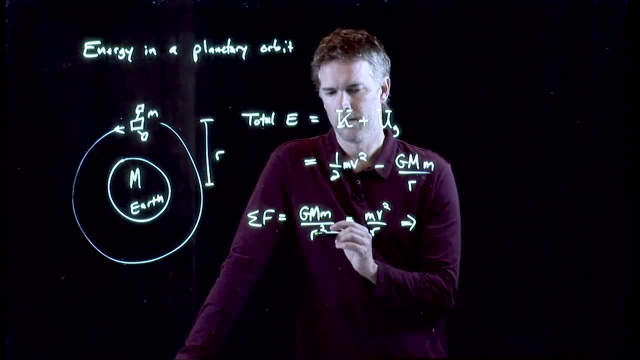 We'll get rid of that. Okay, We'll get rid of that r and we'll get rid of one of those. And then let's multiply both sides by a half, And if I do that, this side becomes one half mv squared. 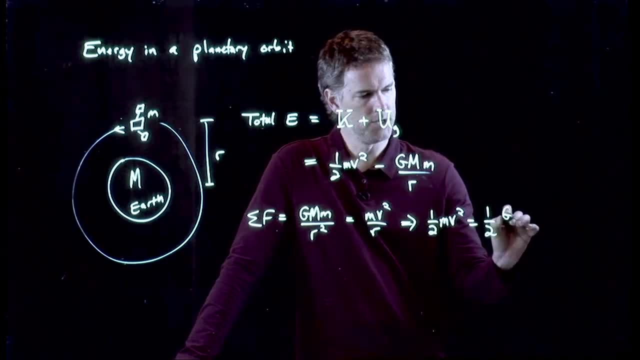 and the other side becomes one half g, m, m over, r. Remember we got rid of one of the r's, so we just have one left. Aha, And this thing we can plug back into this equation, And so the total energy. 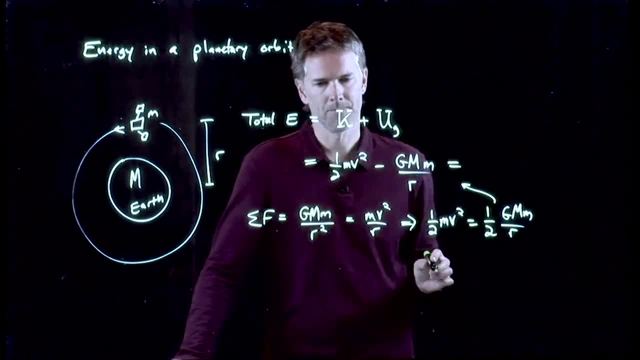 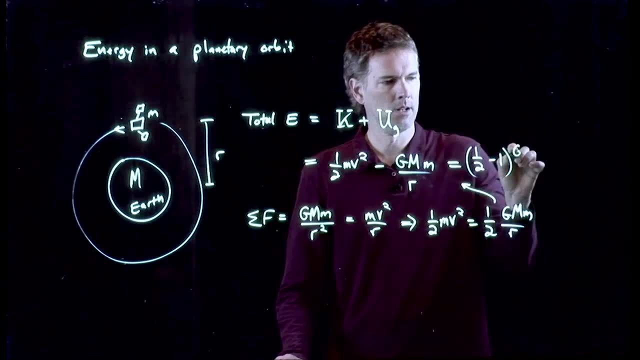 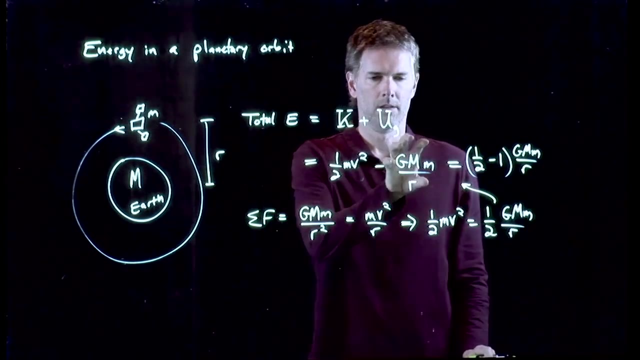 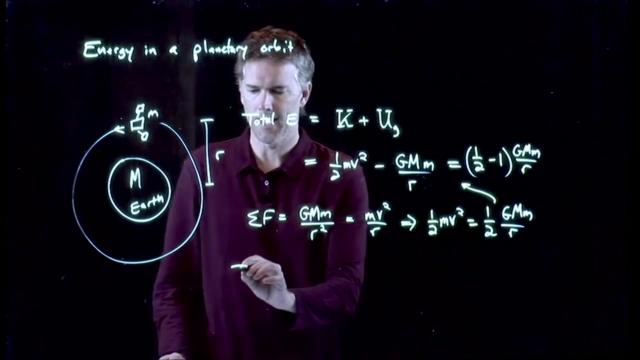 becomes what It is: one half minus one. g m m over r. I get a half from this term That goes here, I get this guy, which becomes the one, And so a half minus one is, of course, negative a half. 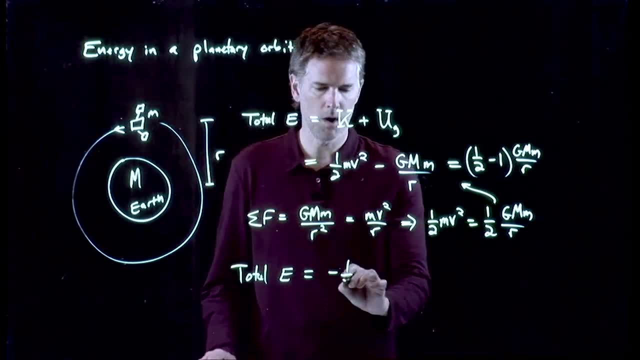 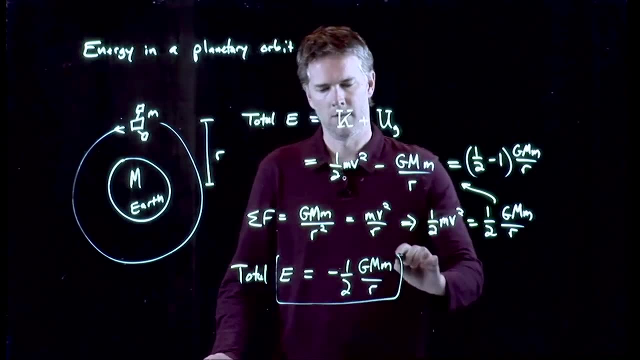 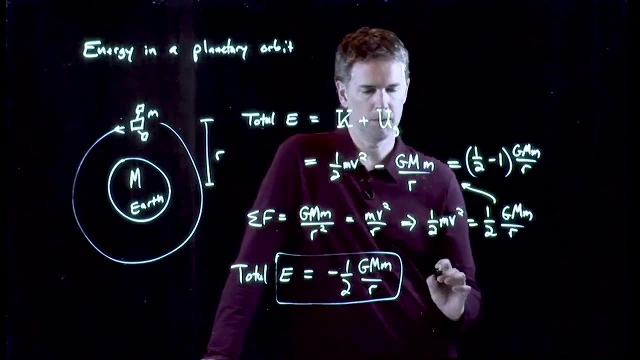 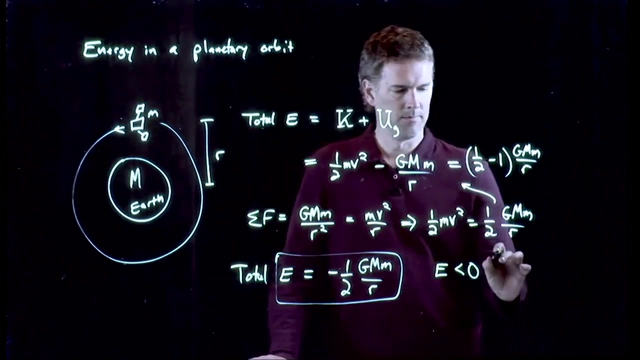 So what's the total energy? It is minus one, One, One half g, m, m divided by r, And those are all positive numbers. And so what's the energy in the planetary orbit, or the satellite orbit? It's negative. We just did a circular orbit. 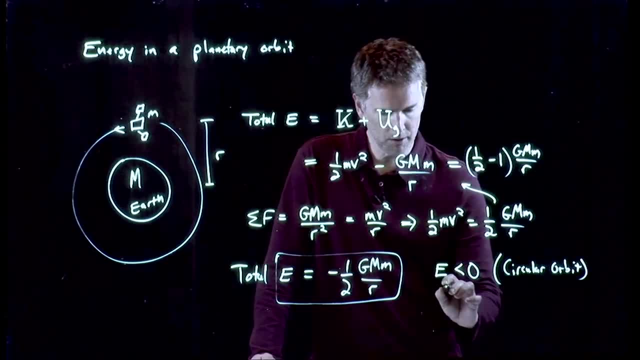 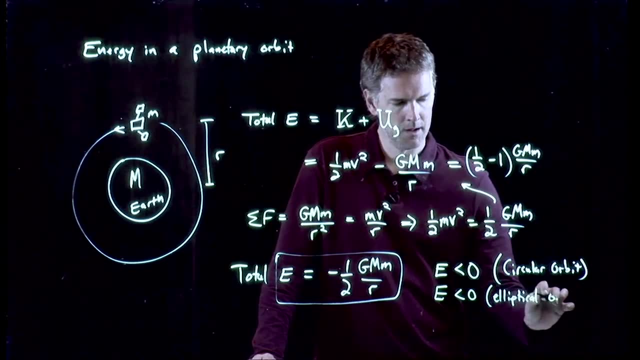 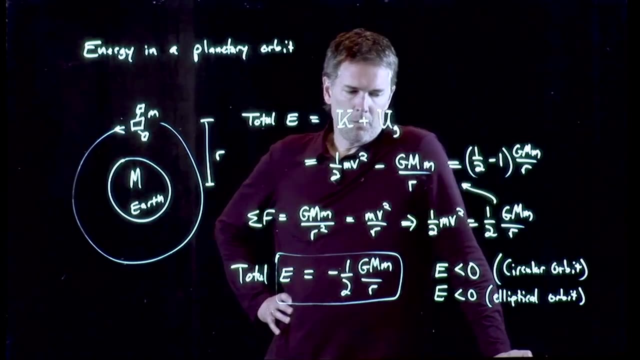 You can in fact prove this Also for elliptical orbits. it's a little more complicated, but the answer is the same: The total energy is also going to be negative for an elliptical orbit. So we're back to this question of negative energy. 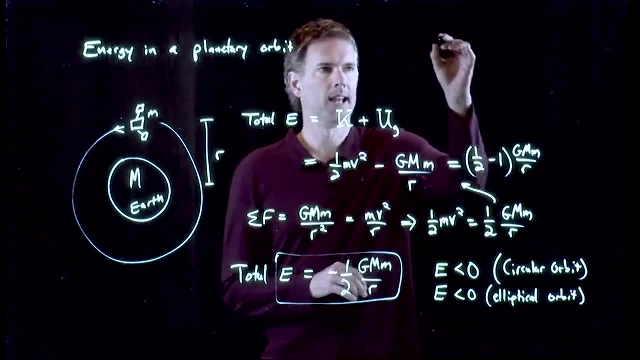 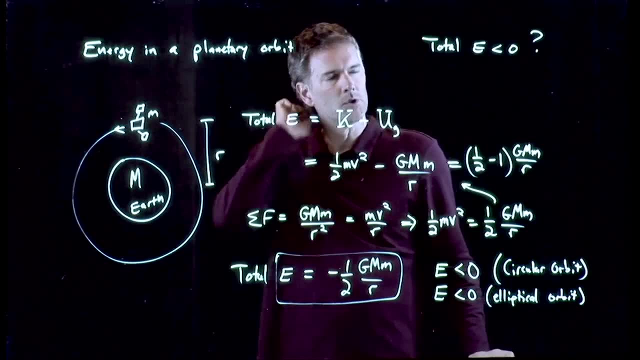 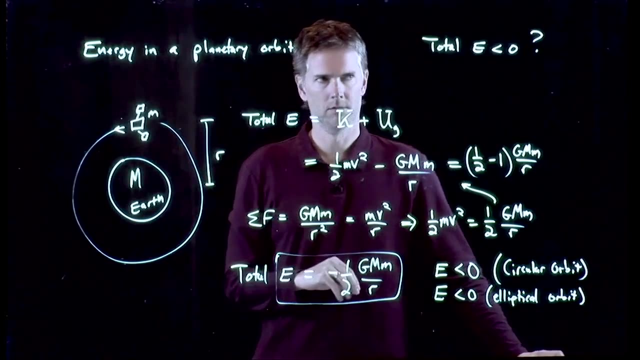 What do we mean by energy less than zero Total energy less than zero Jordan? what do we mean by that? When I say the energy of the system, the energy of this satellite, is negative, what does that mean? It's going to be bound to the earth and never come back. 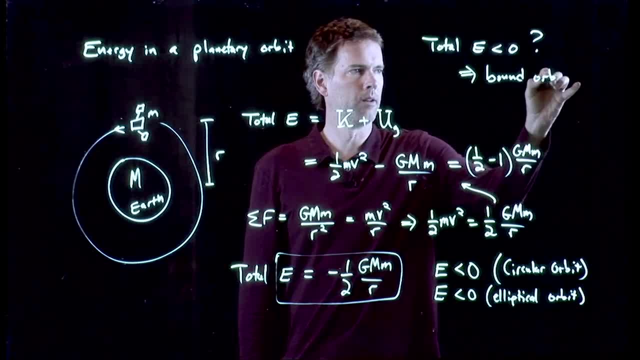 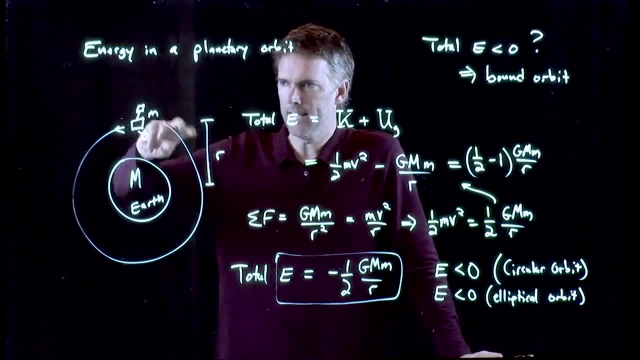 Yeah, that's exactly right. It's a bound orbit. The satellite is bound to the earth through gravity. It can't leave, It can't just fly away into outer space and never come back. It is, in fact, bound to the earth. 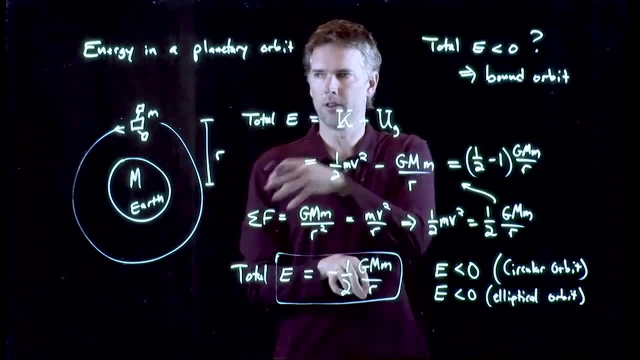 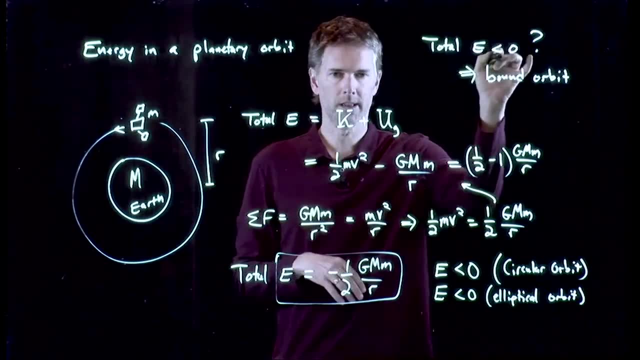 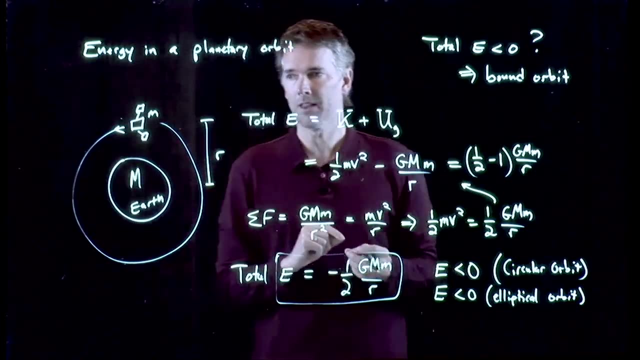 Just like the earth is bound to the sun. Right, We can't fly away from the sun, We are in a bound orbit. Anytime you have a total energy that is negative, that is a bound orbit. And guess what? It doesn't have to be two particles that have mass like this. 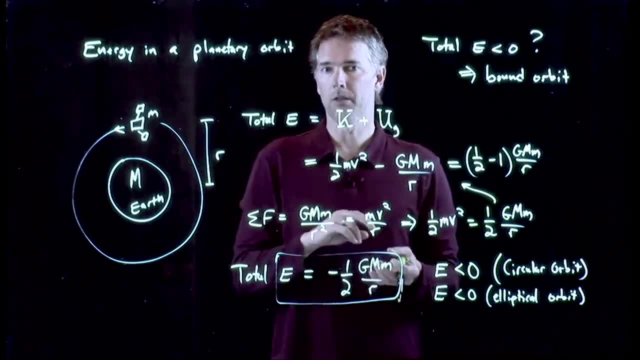 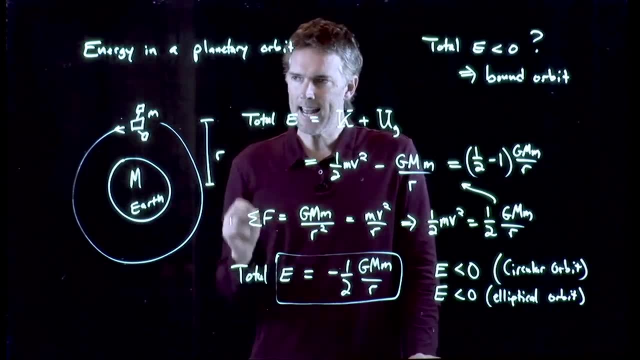 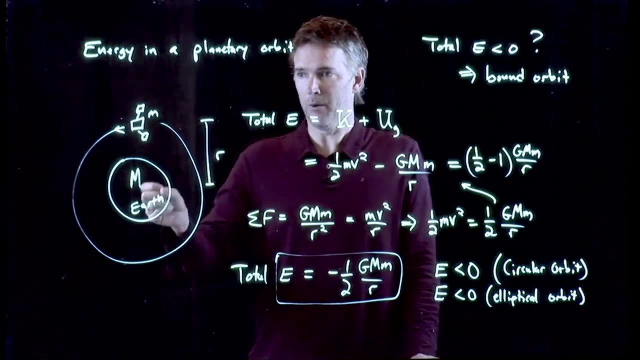 It could be two particles that have charge, like the proton and the electron. The electron that orbits the proton has a negative energy, Negative energy- And that means it is bound, which is a good thing, Because if it wasn't bound it would fly away and we wouldn't have atoms. 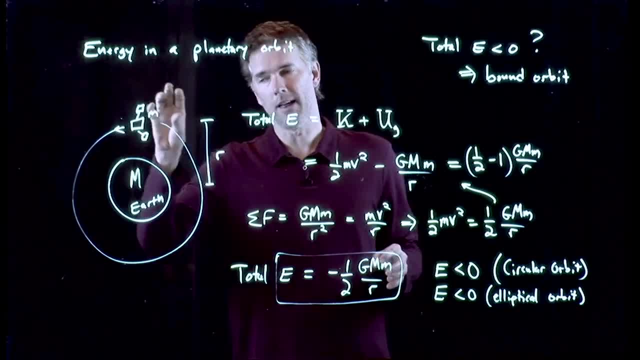 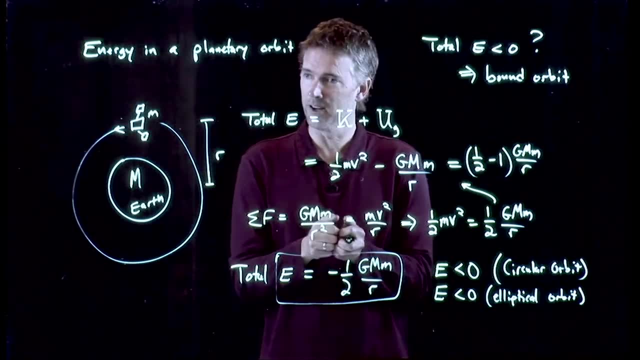 Okay, It's a good thing that we're bound in this case, because if that satellite wasn't bound, it would fly away. We wouldn't have GPS. You wouldn't be able to find the nearest Starbucks, right When you go to your Apple Maps. okay, Or that Loch Ness Monster, Whatever you're looking for.